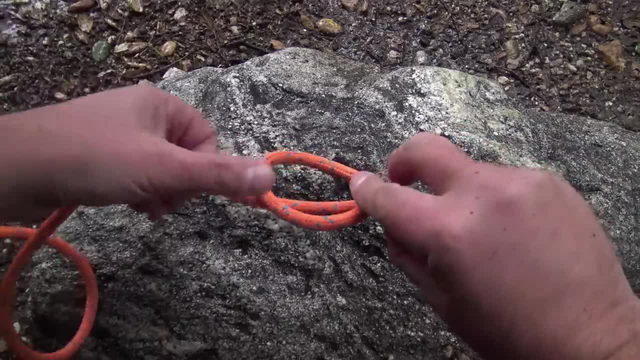 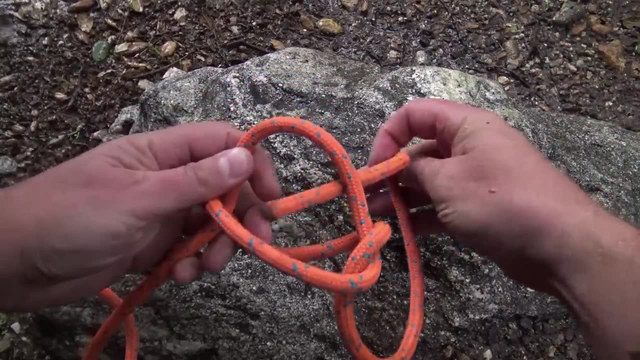 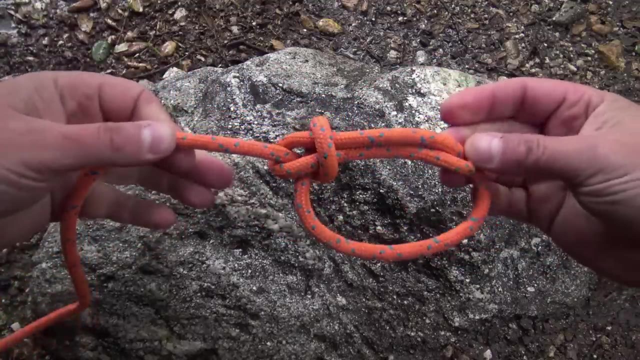 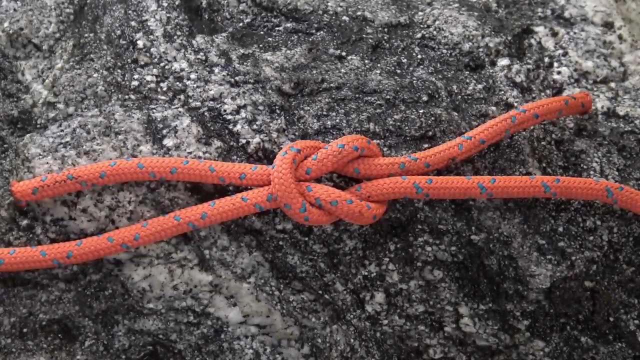 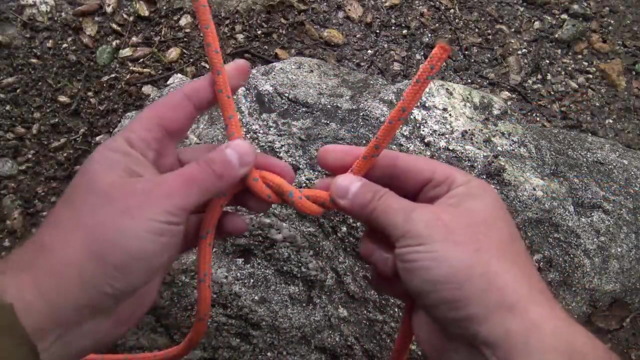 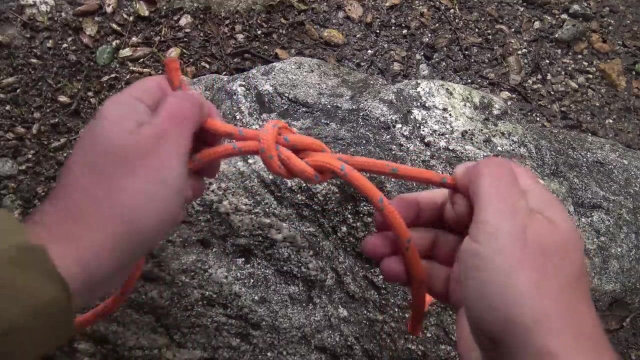 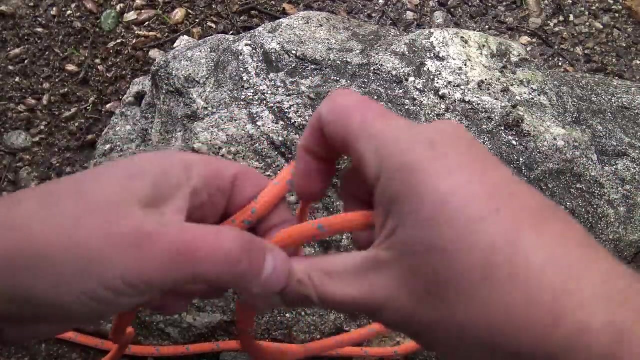 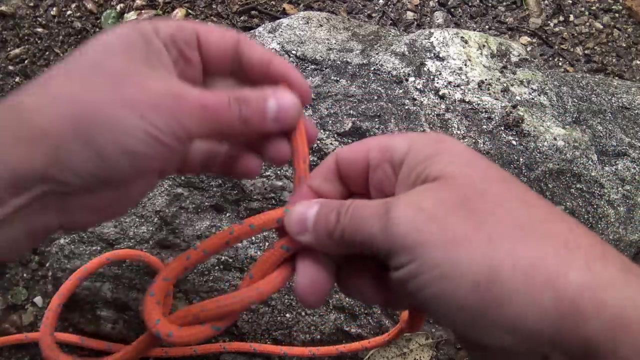 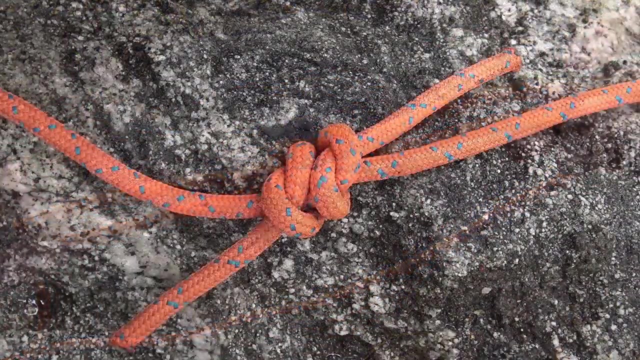 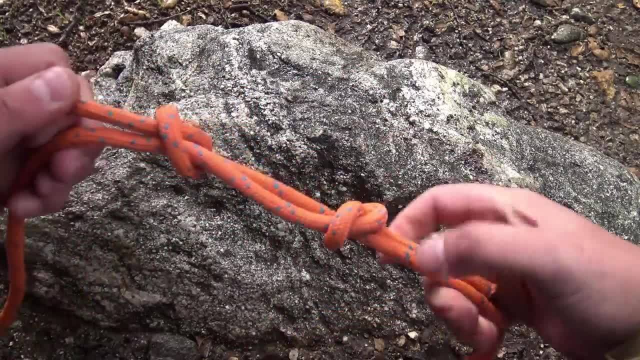 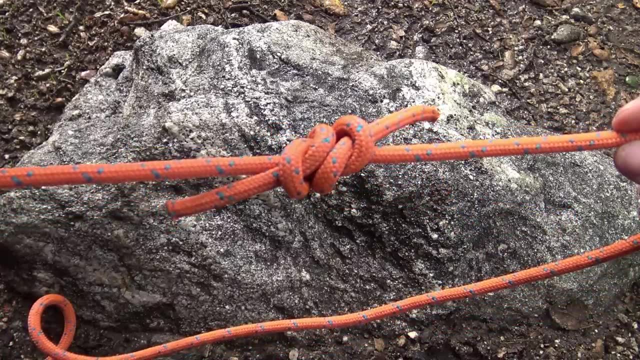 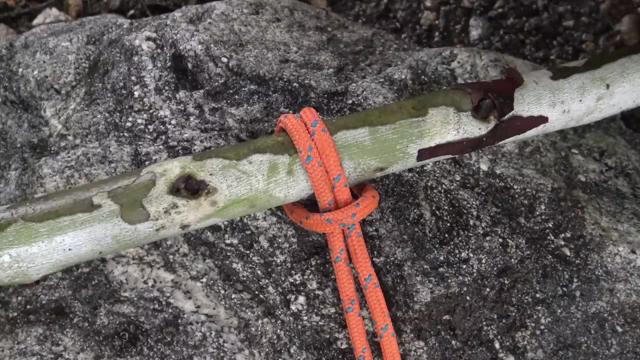 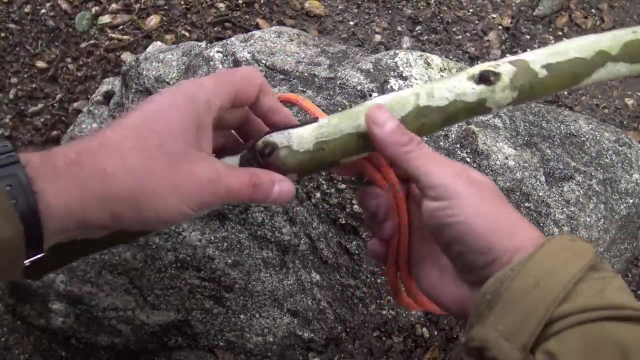 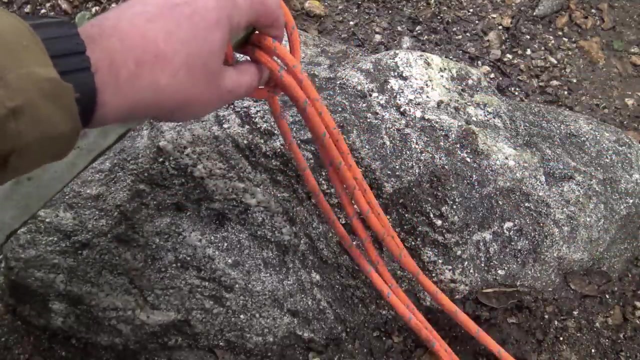 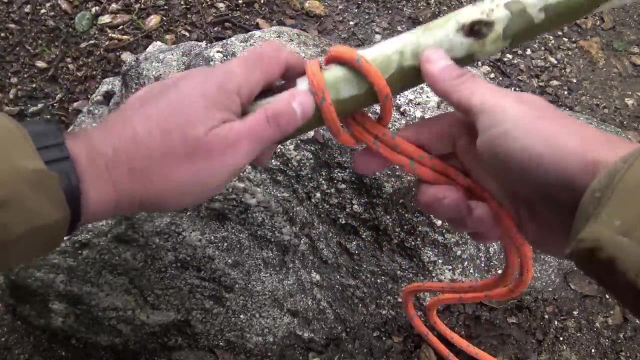 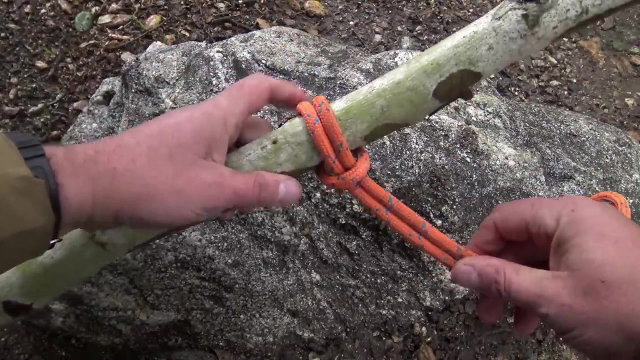 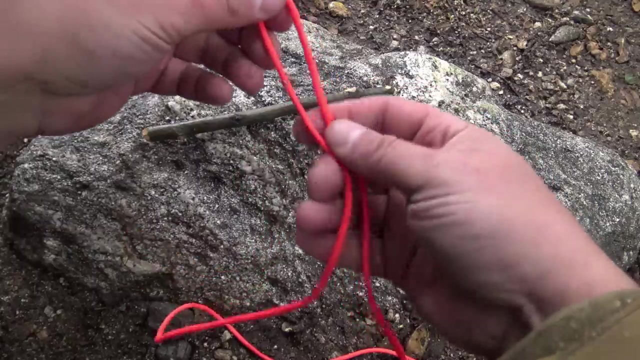 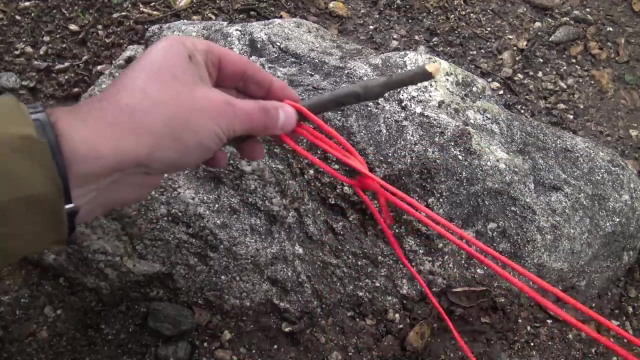 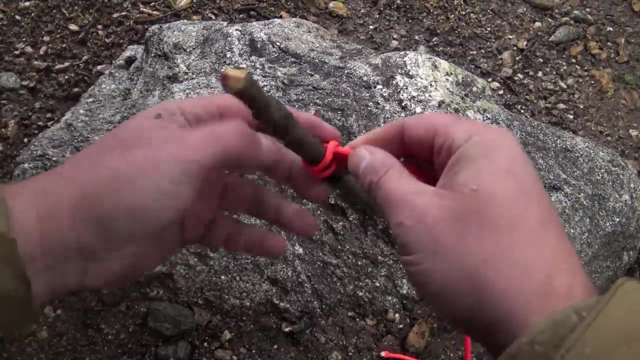 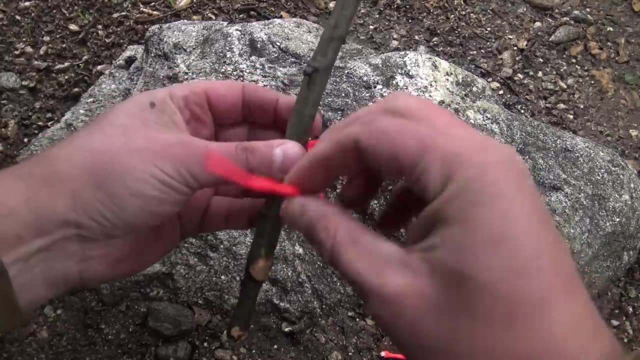 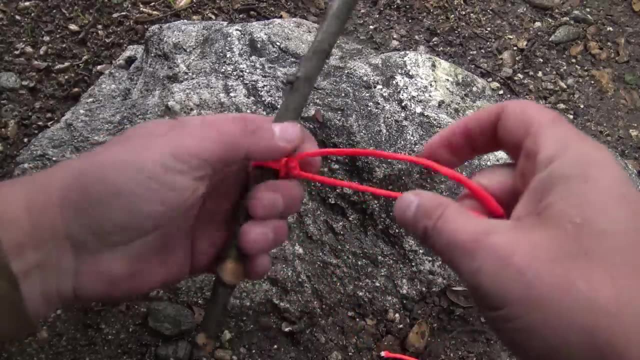 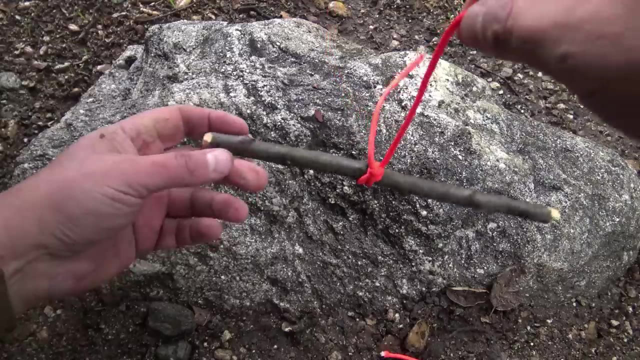 A lark's head knot, sometimes referred to as a cow hitch, can be used to attach a piece of cordage to an object. A lark's head knot can be used to attach a piece of cordage to an object. A lark's head knot can be used to attach a piece of cordage to an object. 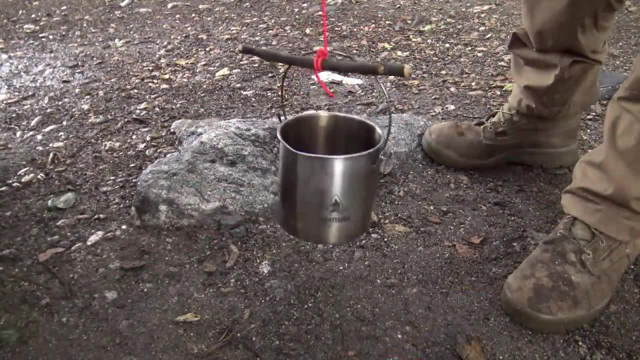 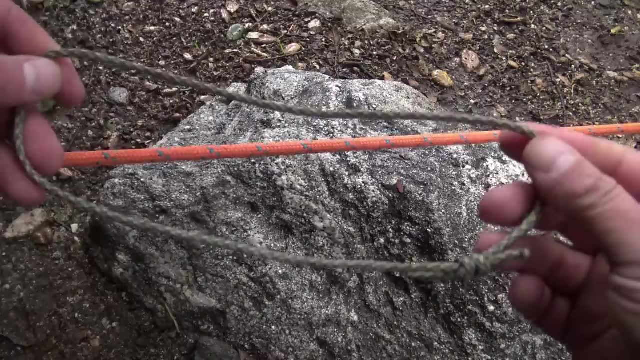 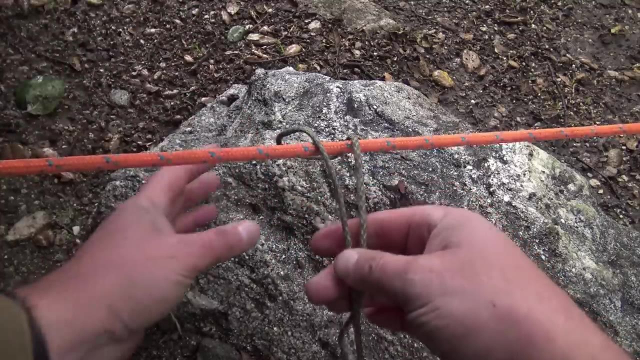 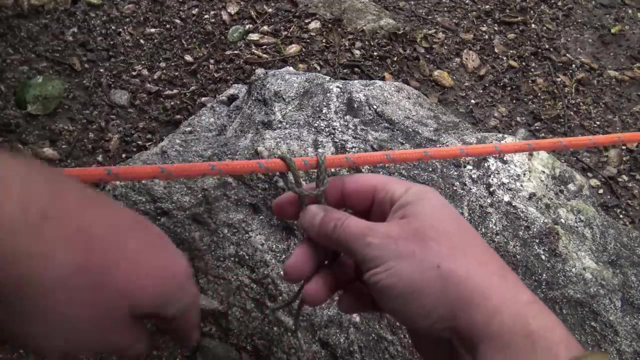 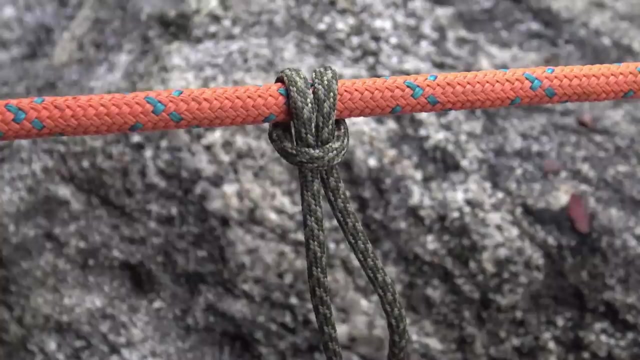 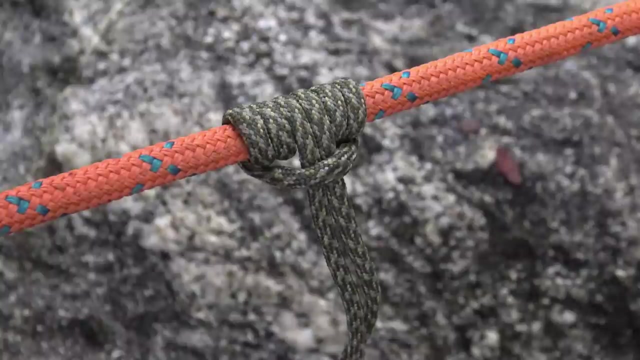 A lark's head knot can be used to attach a piece of cordage to an object. The Prusik knot is perfect for attaching a loop of smaller diameter to a larger diameter rope. The beauty of this knot is that you can slide it in either direction. 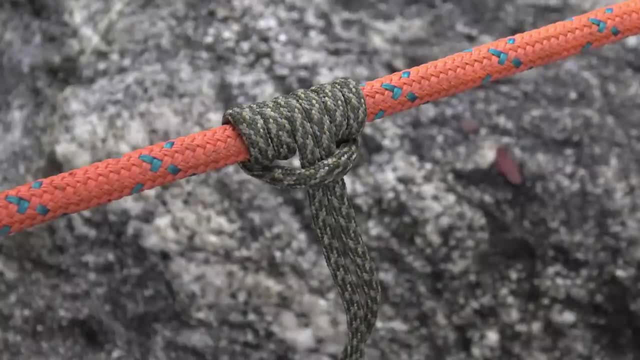 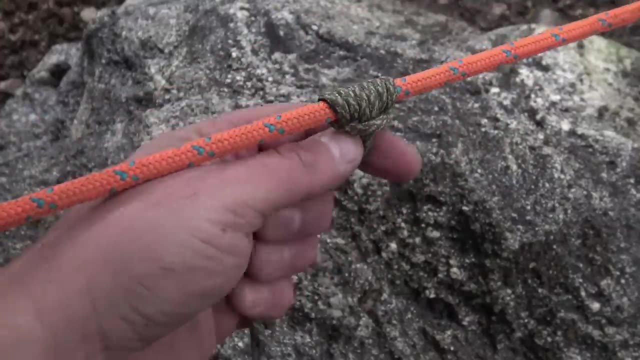 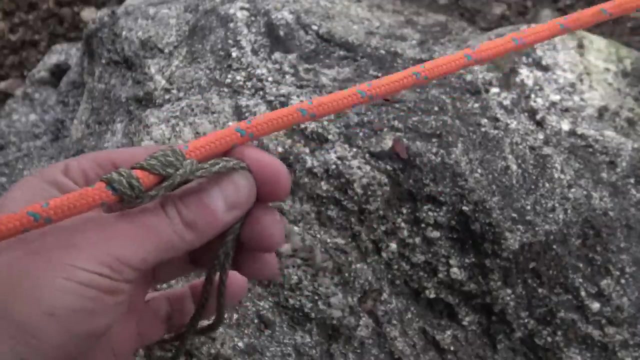 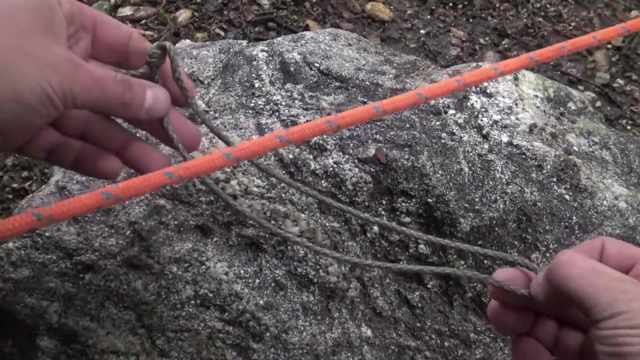 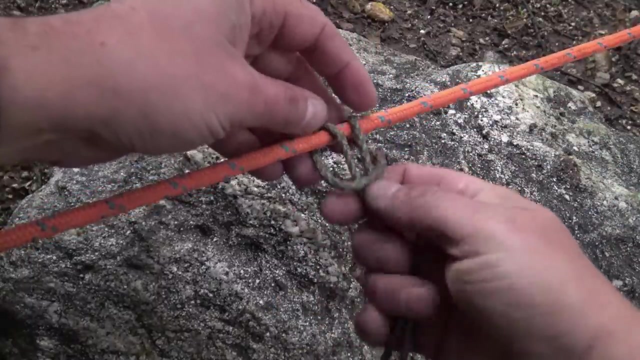 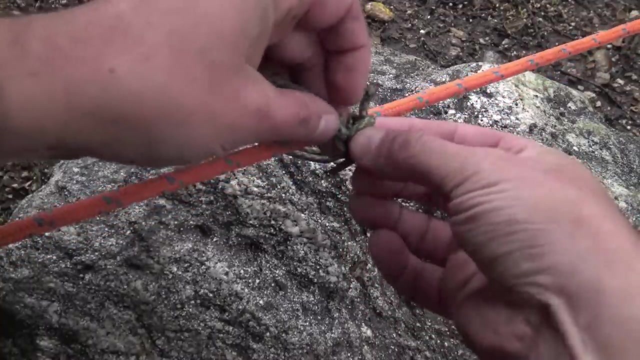 but once you pull in the opposite direction it will lock in place. The sit or hook type knot can be used to attach a string or frame to the knot. For effortlessnatuities, this knot will often have to be attached to a pulling rope. 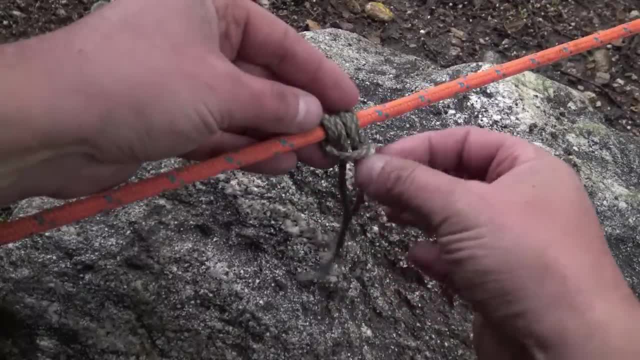 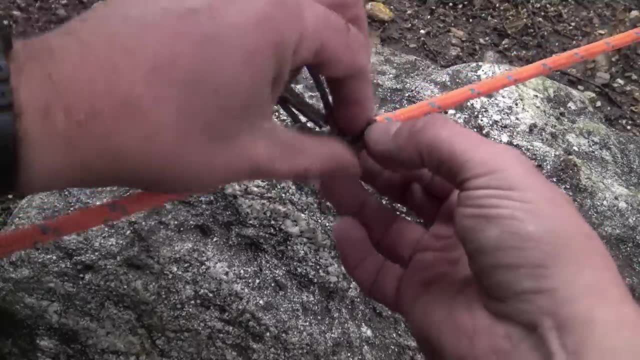 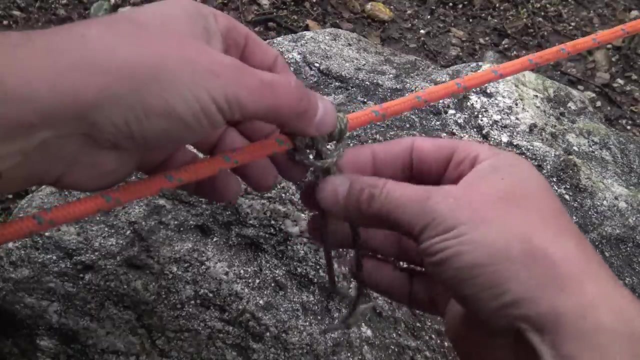 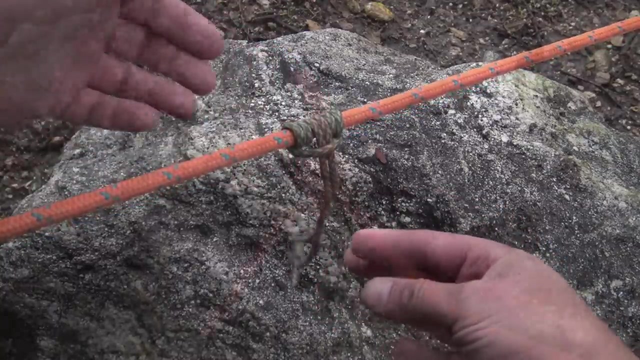 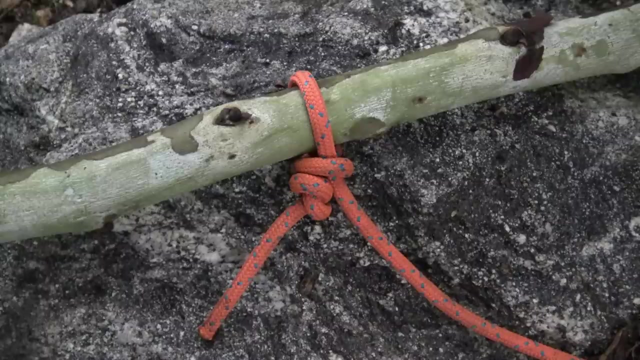 You may notice that the knot is rather loose, but that's ok. Yes, The jam knot, sometimes referred to as an arbor knot, can be used to compress a load, the lashing, or simply tie a piece of cordage around an object. 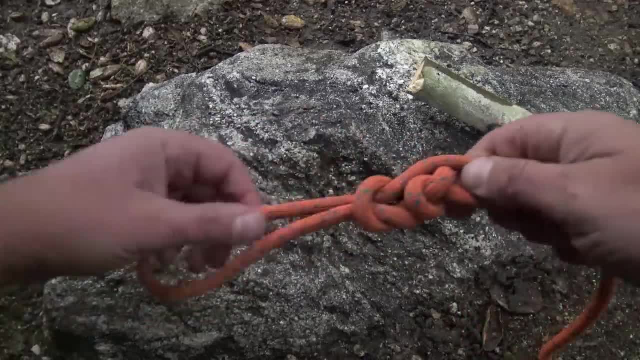 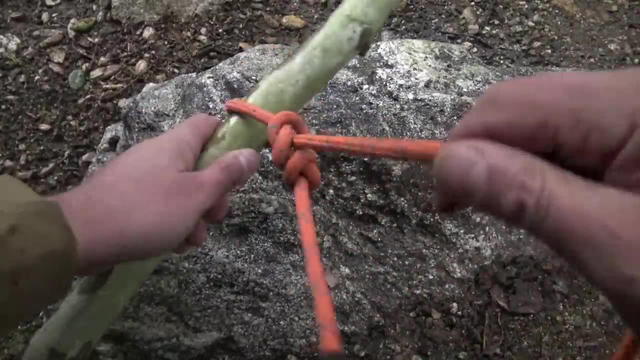 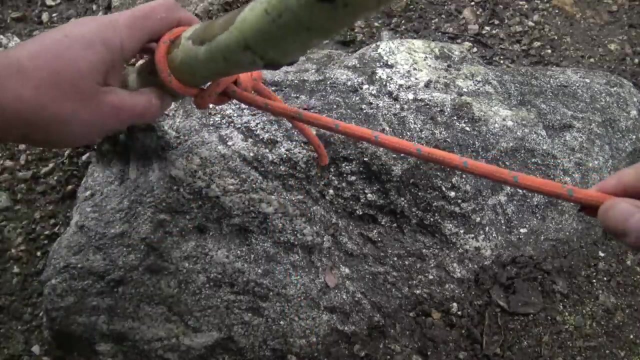 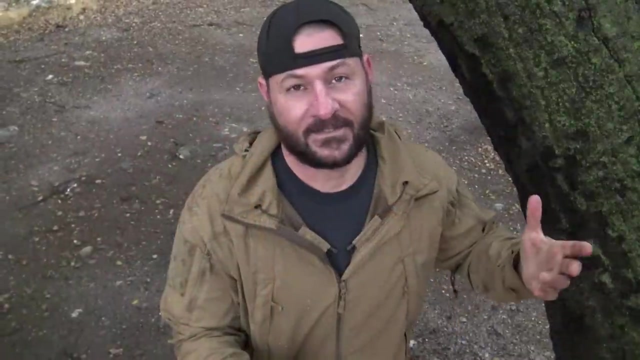 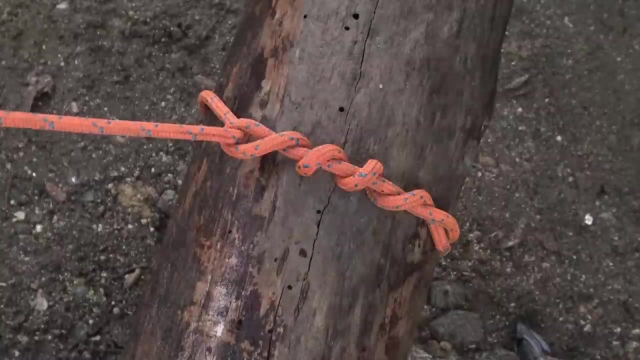 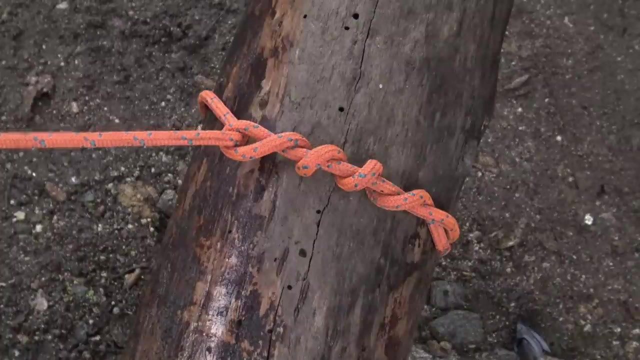 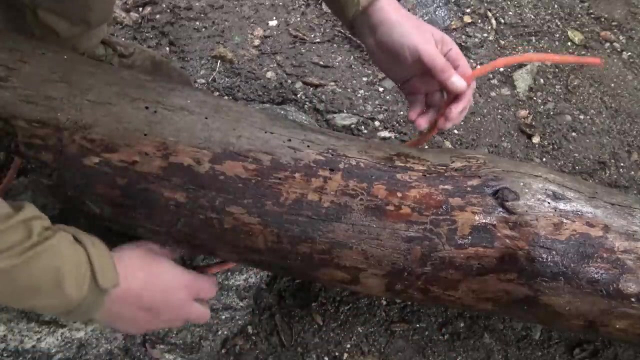 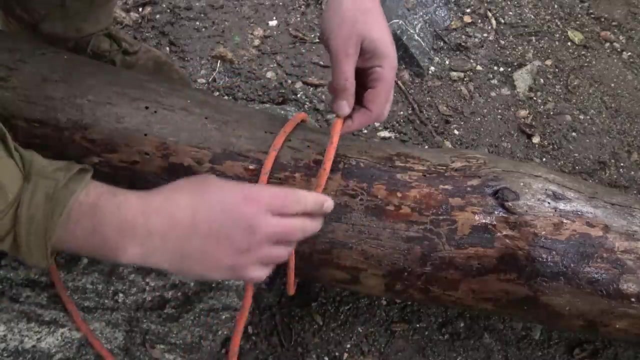 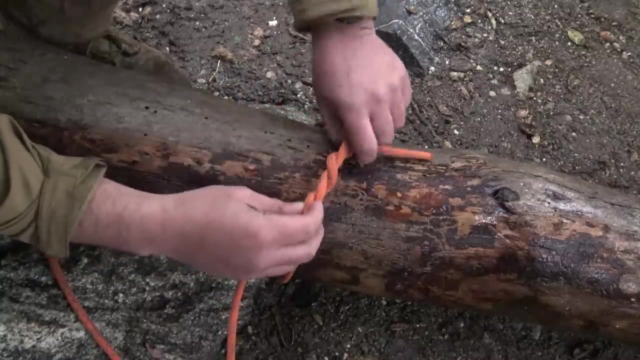 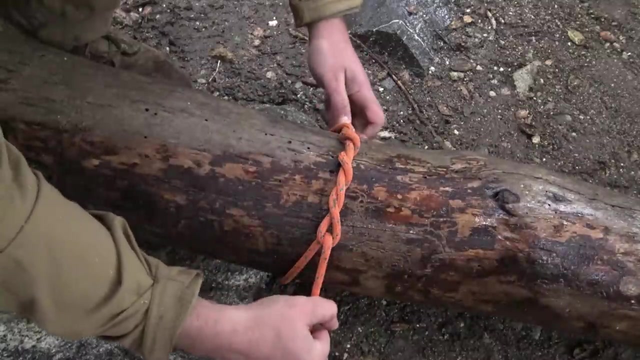 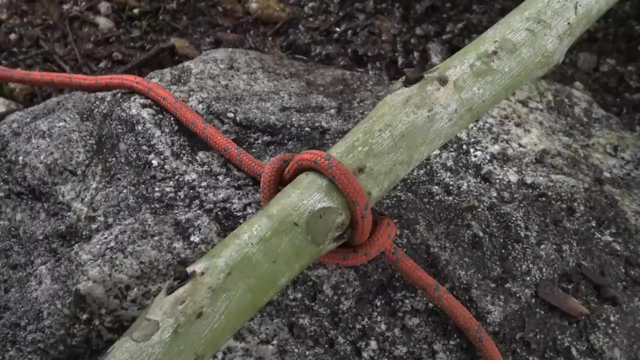 As always, if it ain't raining, we ain't training. Let's go ahead and move into some essential camp hitches. A timber hitch can be used when towing a log tree or even starting a lash. A marlin spike hitch is a temporary knot used to attach a rod to a rope in order to 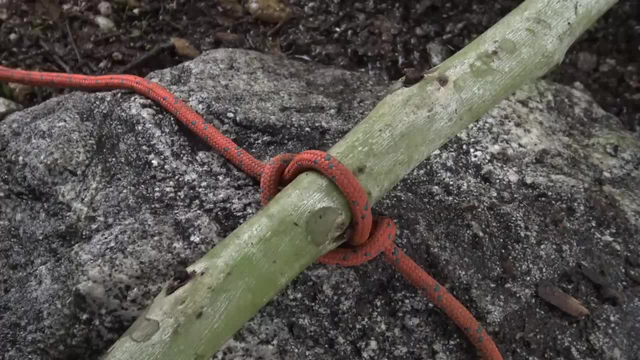 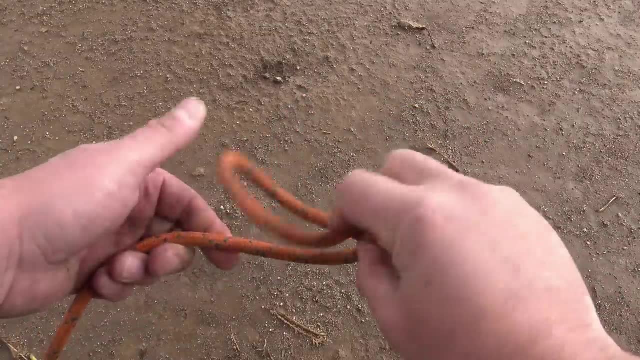 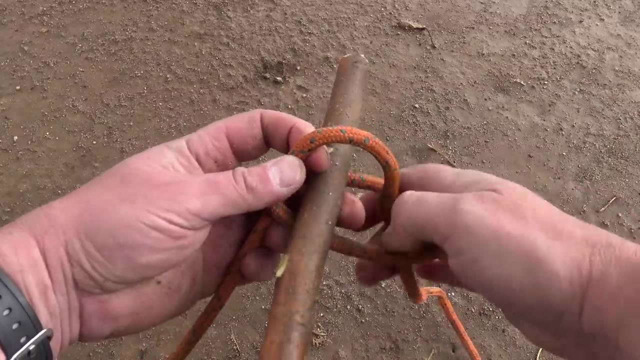 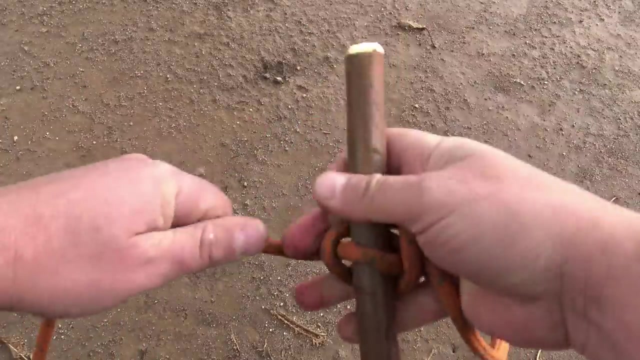 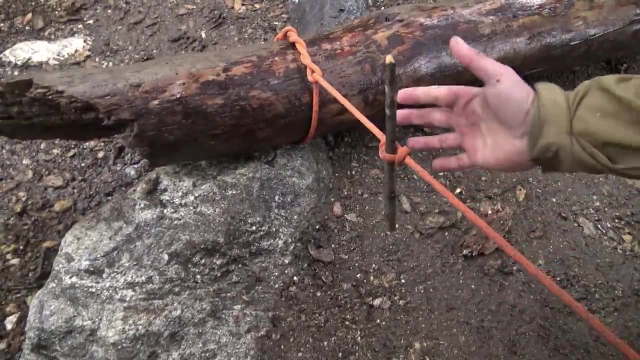 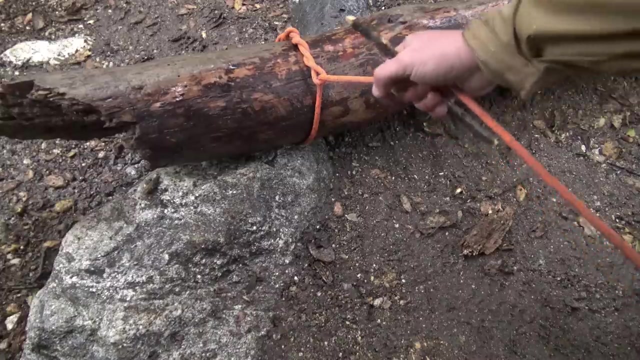 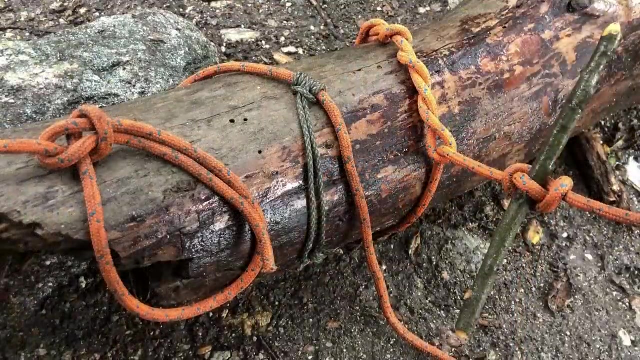 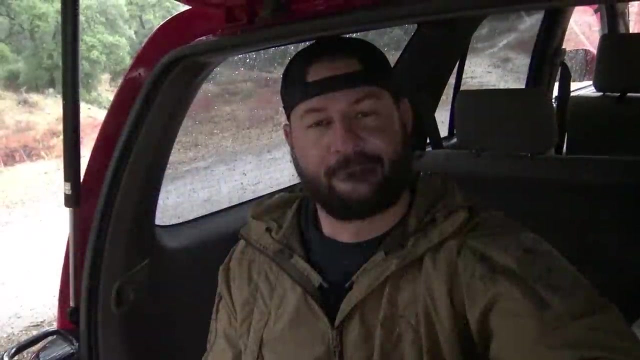 form a handle or rung for a ladder. It's great, Oh No, And by simply combining the two, I have my Marlin spike hitch T-handle, my timber hitch around that log and I'm in business. Welcome back. 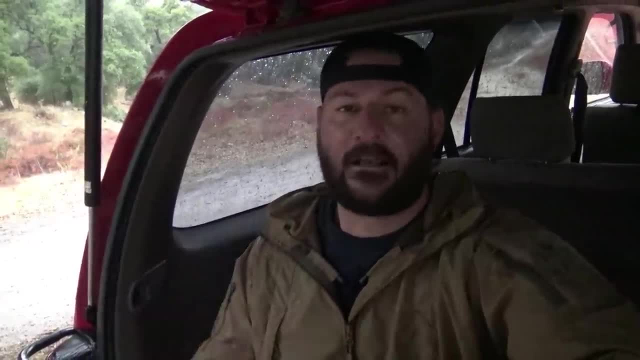 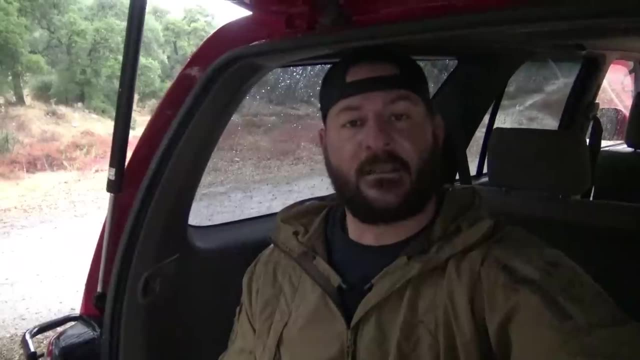 Camp knots and hitches will make your life outstanding and a hell of a lot better as well. As always, all the gear in my videos can be found on my Amazon Influencer page. I'll toss that link inside the description box. Please do me that favor. 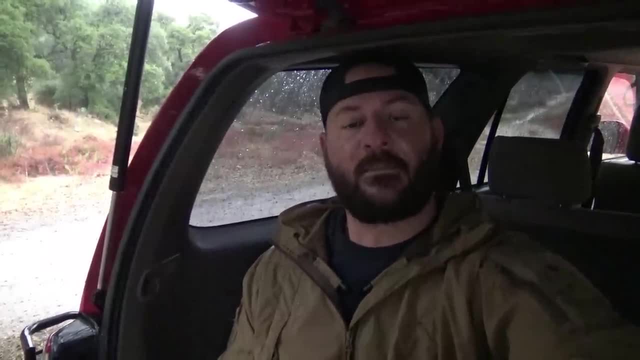 Hit that like and subscribe button. Then ring that notification bell. Once you ring that bell, please select all notifications And, as always, thank you for your comments, views and support. Thanks for watching. Get out in the field and have some fun. 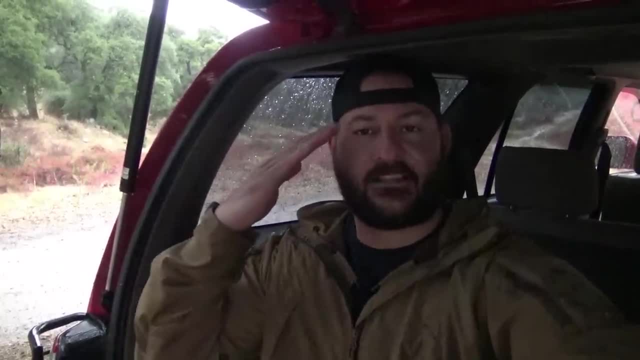 I'm going to catch you next time.